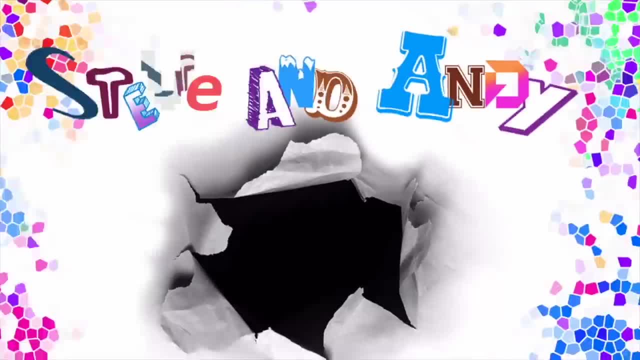 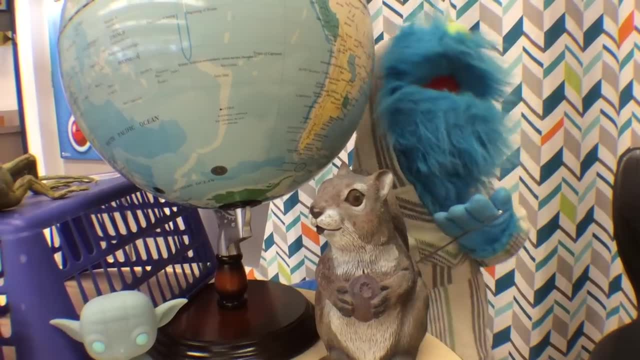 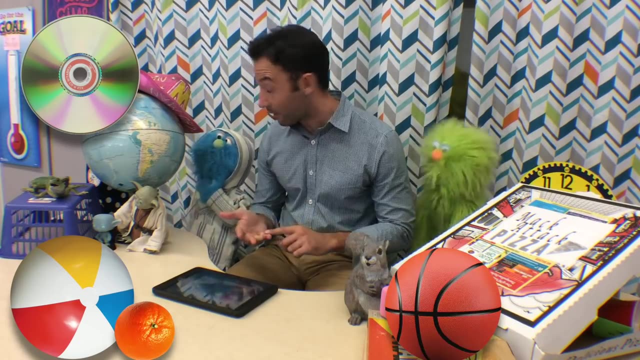 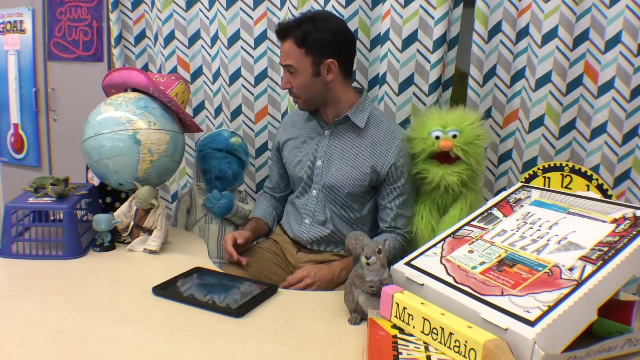 All right, so I'm gonna give you guys a hint about our next topic. Okay, go. A CD, a beach ball, an orange, a basketball- Oh, is it jean shorts? How'd you get jean shorts from a CD? a beach ball, an orange and a basketball? Well, they're all things I keep in my jean shorts. No, they're all rounds. 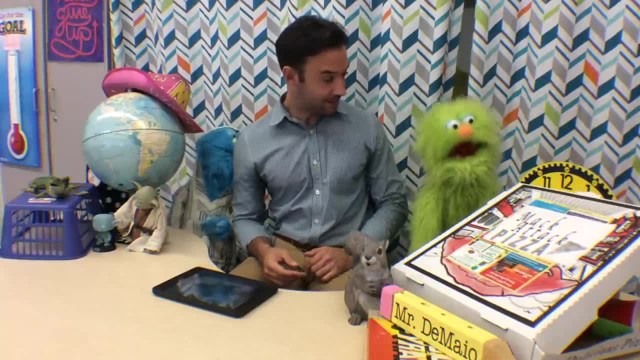 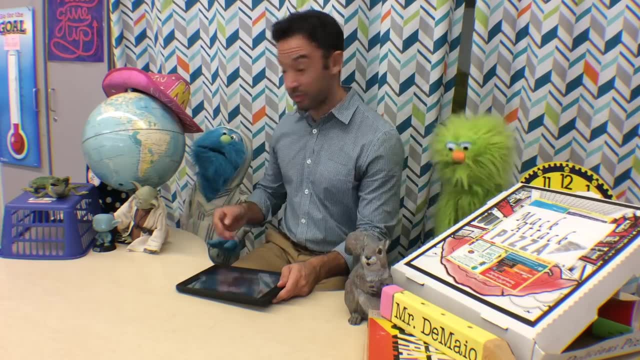 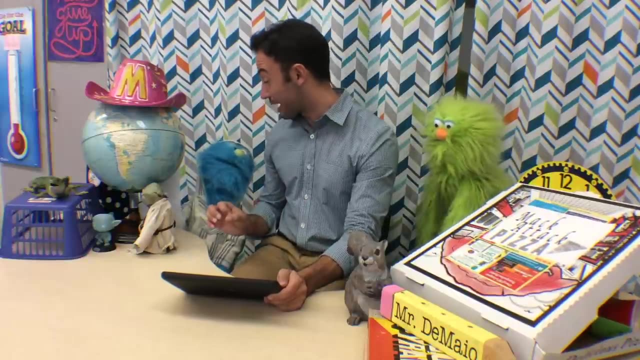 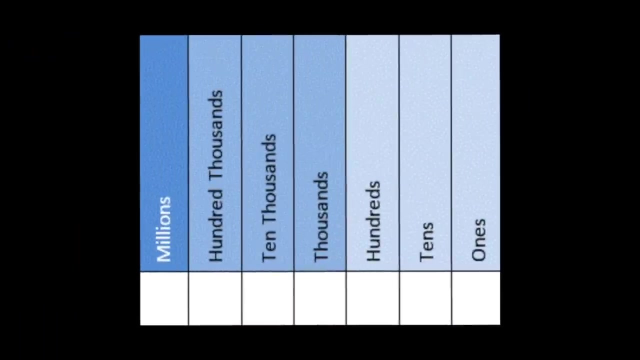 Do you get it Rounding? Oh, I get it. It's a horrible joke, but I get it. Well, I may joke around now. Rounding is no joke at all. It's something that's used in math all the way up through college, So I guess I should pay attention. huh, Yes, totally. Now the first thing you need to know in rounding is place value. Some kids may know it already, but let's just review it really quick. This is a place value chart. It tells the value of each number. So let's say, if you write the number 128,, 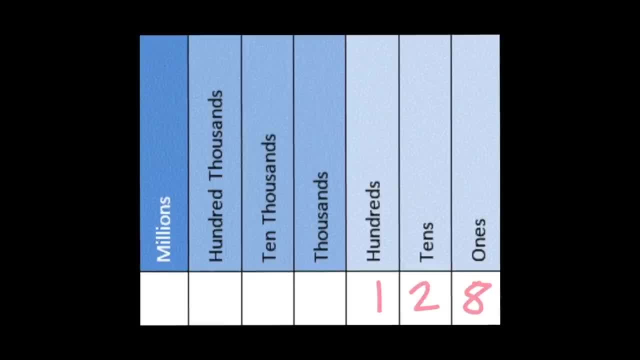 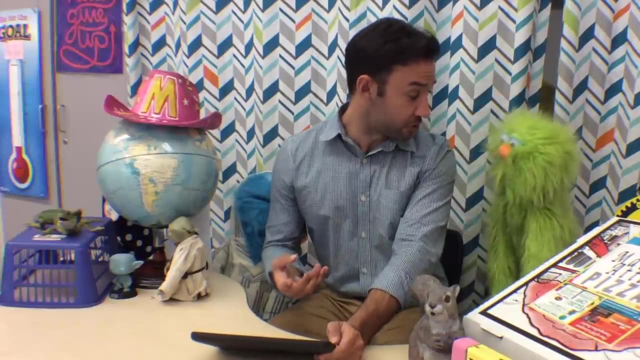 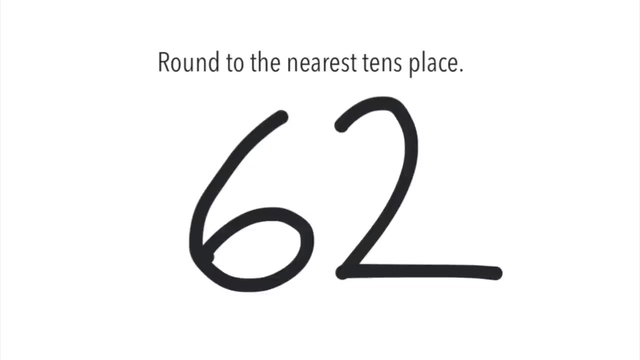 the 8 is in the 1's place, the 2 is in the 10's place and the 1 is in the 100's place. You're going to need to know place value if you're going to round. What does place value have to do with rounding? Well, it's all in the directions of the problems you're reading Here. look at this. Take a look at the problem here. The number is 62.. Now take a second to read the directions above it. They say round to the nearest 10's place. So, Andy, 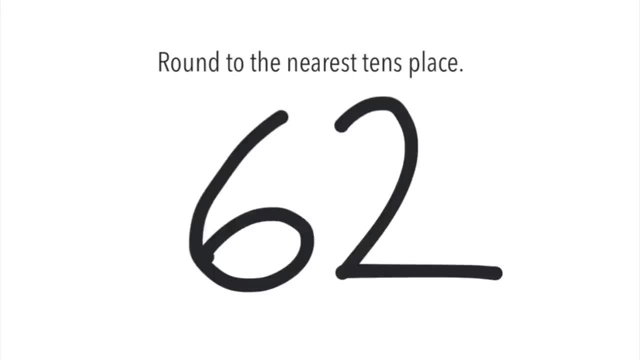 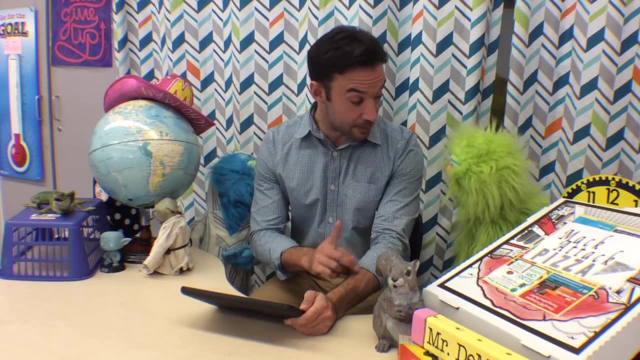 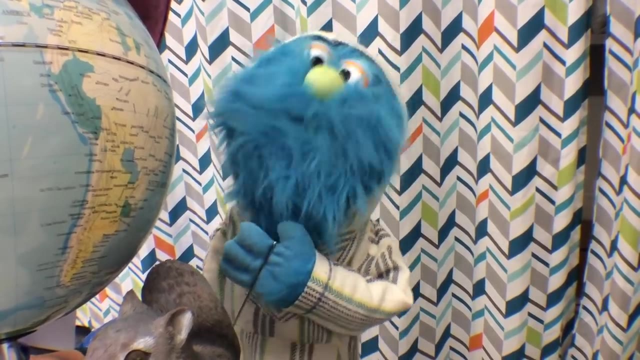 using what you learned before. what number is in the 10's place The 6?? Correct, We're making progress now, but the first step is to underline the number you're working with Here. go ahead, say it Under, where the number you're working with Not even close. Try it again, Underline. 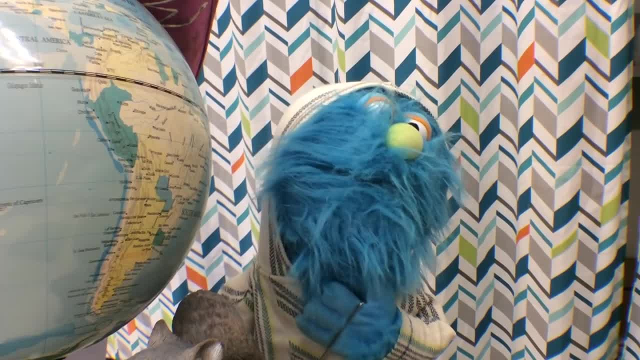 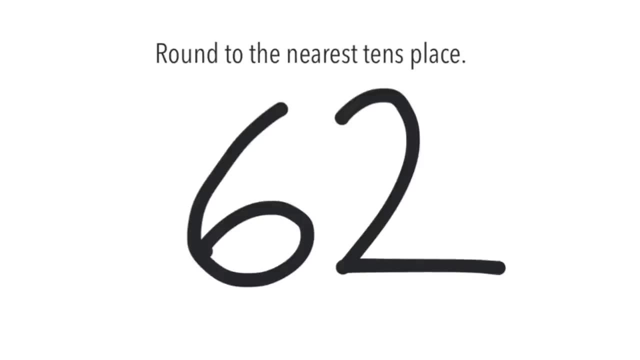 the number you're working with, Correct. So if it says round to the nearest 10's place and you're supposed to underline the number you're working with, well, what number should we underline? The 6. Correct, Okay. so what's next? Well, the next thing I say is to circle. 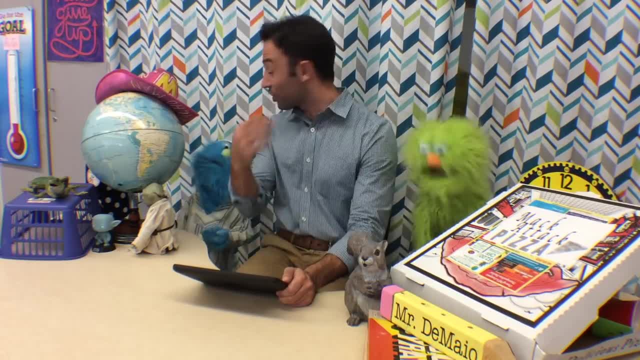 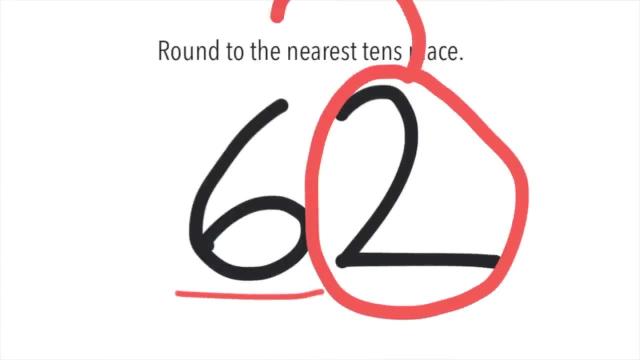 the number next to it Here. say it with me, Circle the number next to it. So we circle the number next to it and this number affects this number tremendously. Now you ask yourself a question: Is the number you circled closer to 10 or 0?? It's definitely closer to 0. Yep. 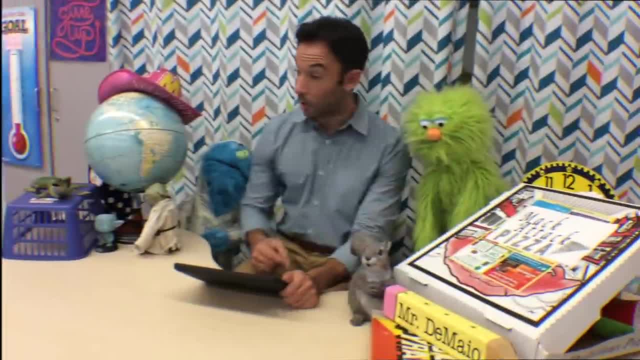 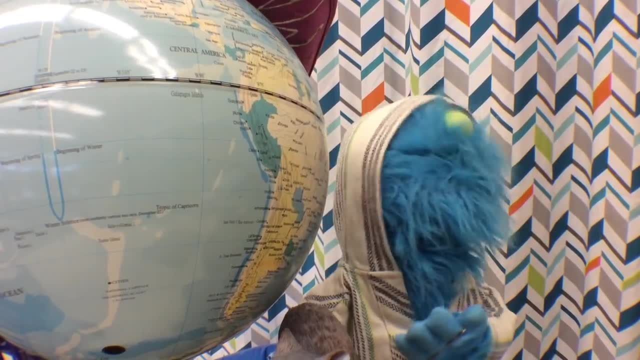 so we turn it into a 0, and we're done All right. so what's the answer? Is it 60?? Ding, ding, let's continue. But what if the number you circled is closer to 10?? Let's try it. 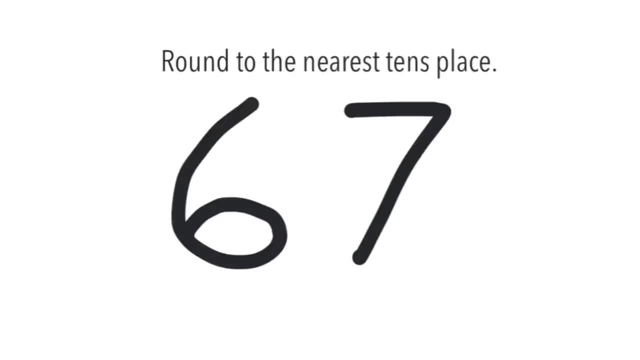 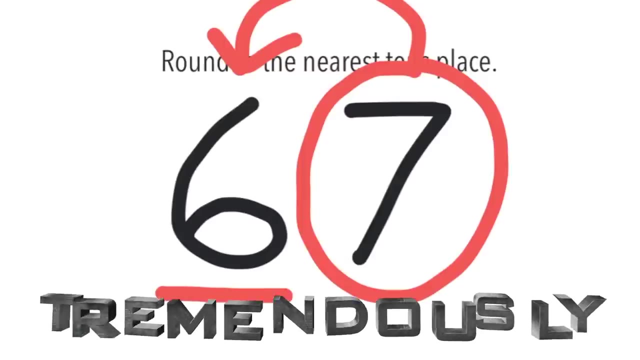 So let's repeat the steps, This time the number 67.. The directions say round to the nearest tens place. So what do we do? Underline the number you're working with, Circle the number next to it. This number affects this number tremendously. Now you ask yourself a question: Is the number? 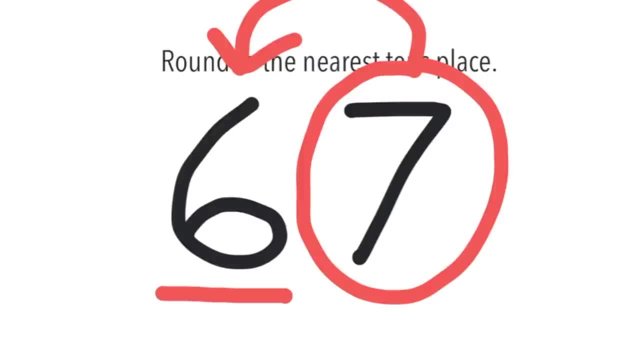 you circled closer to 10 or 0?? If it's closer to 0, you turn it into a 0, and you're done. But the number we circled is 7.. Is that closer to 10? It's closer to 10.. Correct, So we turn the number we circled into a 0, and the other number goes up. 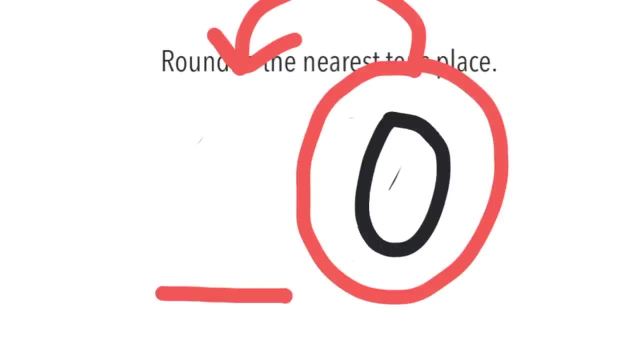 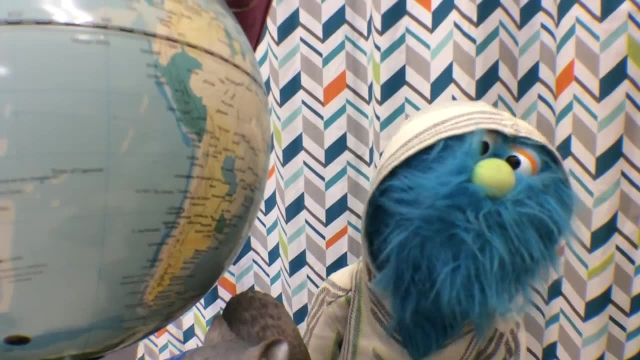 by 1.. So what's one number higher than 6?? Is it 7?? Bingo, and you're done All right. so let's repeat the steps. Step brothers, step up to the streets, step by step. the stepford wives No. 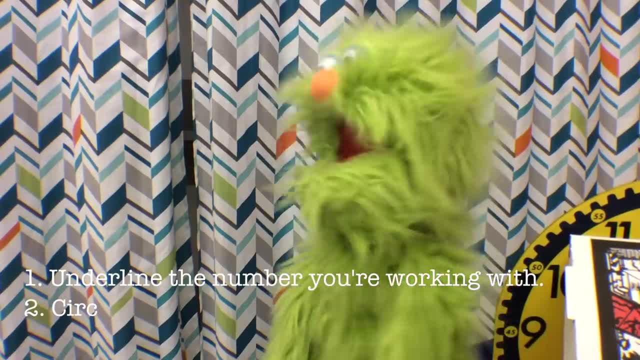 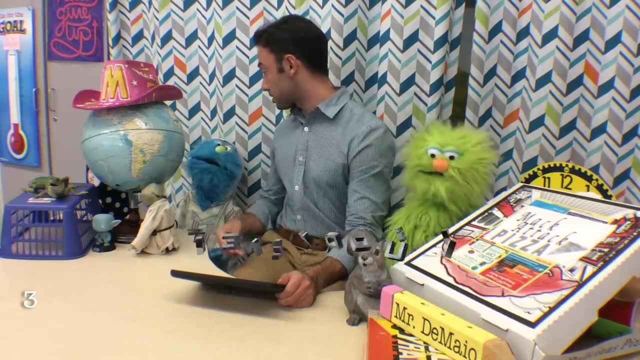 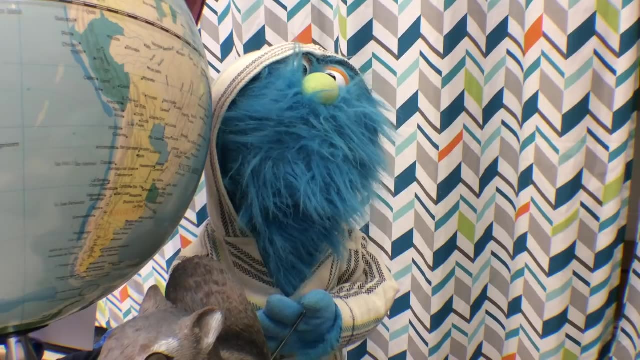 try again. Underline the number you're working with, Circle the number next to it. The number you circled affects the other number tremendously. Now you ask yourself a question: Is the number you circled closer to 10 or 0?? If it's closer to 0, you turn it into a 0, and you're done. 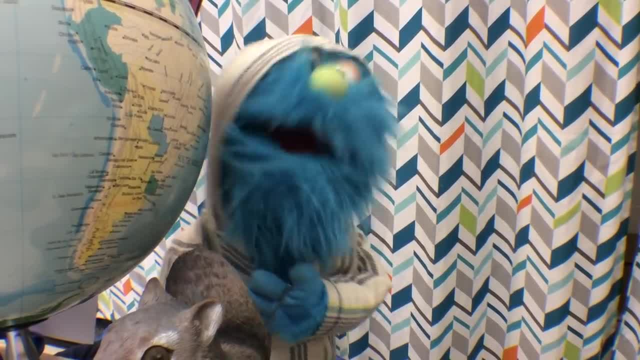 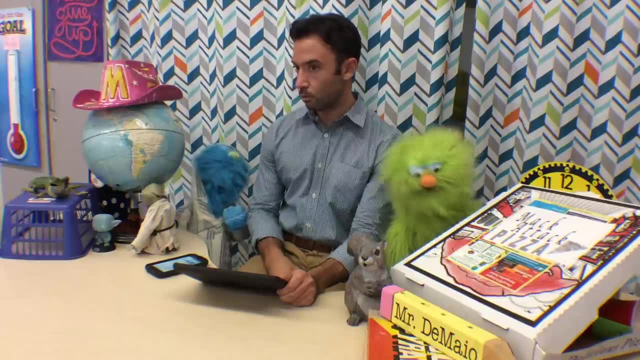 But if it's closer to 10, you turn it into a 0,, but the number you underlined goes up by 1.. It's that simple. But what if it's a bigger number, like 237? Well, you still follow. 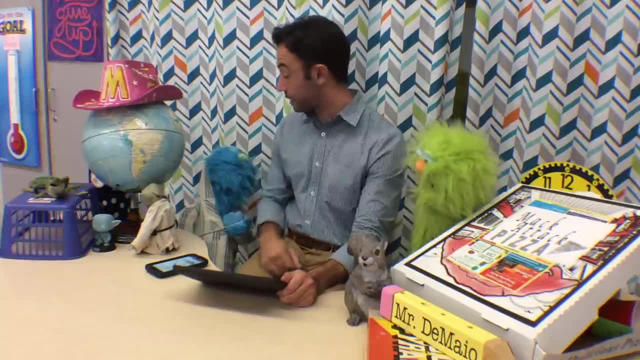 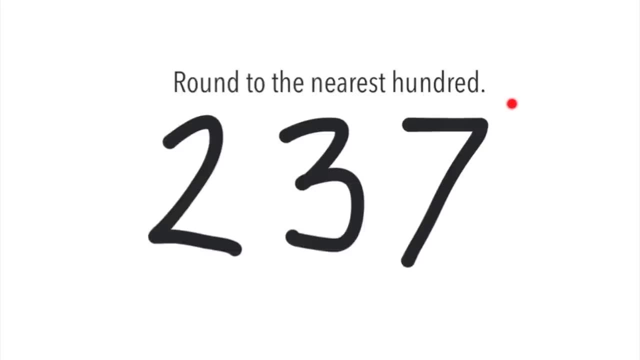 the same steps, but there's one extra rule Here. look at this. So once again, we look in the directions. This time it says to round to the nearest hundred. So what number is in the hundreds place? The 2? Yep, So the next step is to underline the number you're. 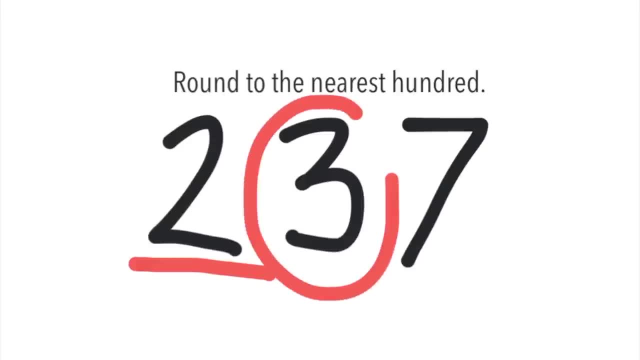 working with. Then we circle the number next to it. This number affects this number tremendously. Now we ask ourselves a question: Is the number you circled closer to 10 or 0?? Well, it's closer to 0. So we turn it into a 0, and the 2 stays the. 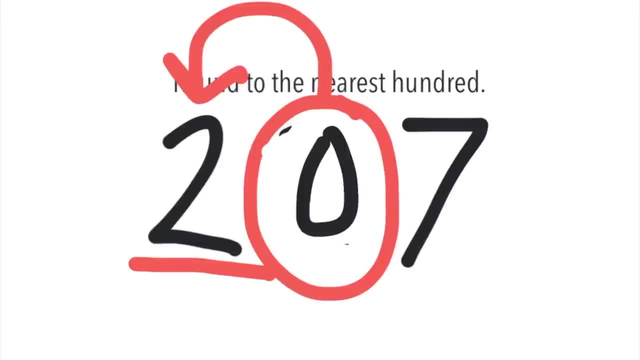 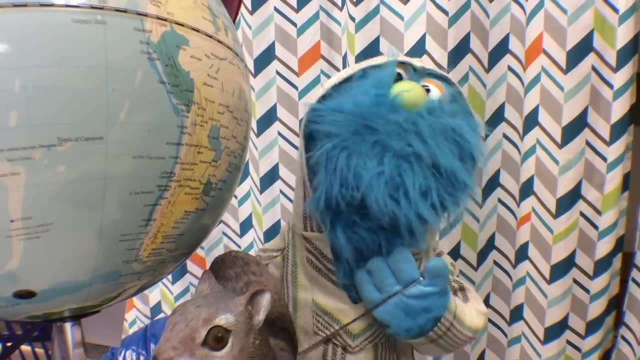 same, But we're still left with that 7.. So we take that number and we turn him into a 0. But why, But, why, what? But why do we turn the 7 into a 0?? Because… He's so lonely. What. 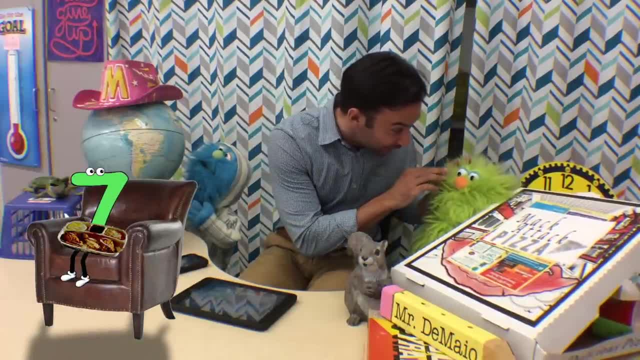 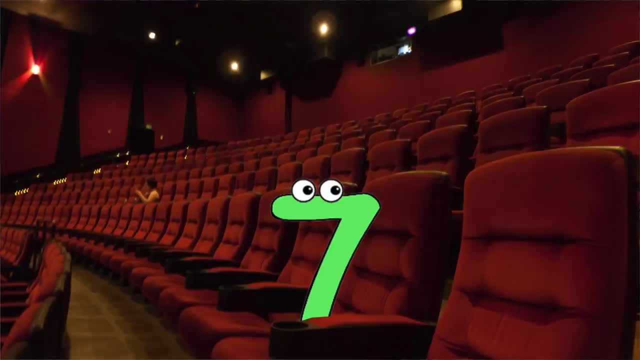 He sits there all alone at night and he eats a TV dinner all alone at night because he's so lonely. I think he's losing it… He goes to the movies all alone and he's so alone and he gets one seat. and troisième, 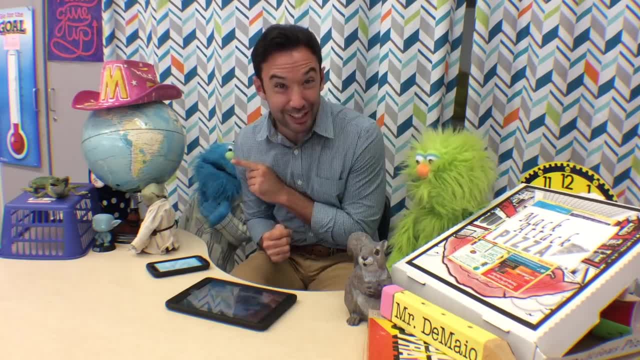 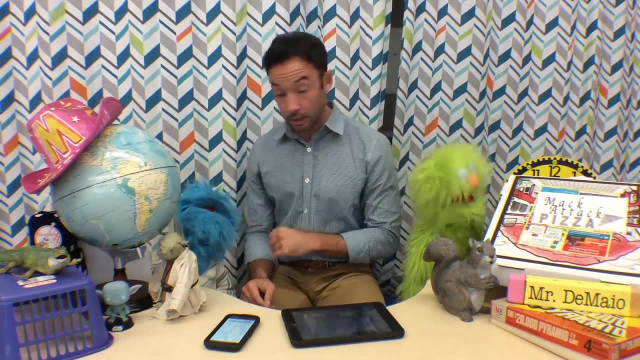 and one popcorn, because he's so lowly. So anything to the right of the number you circled turns into a zero. Yeah, pretty much, but do you know why? Oh, here we go. Because he's so lowly. 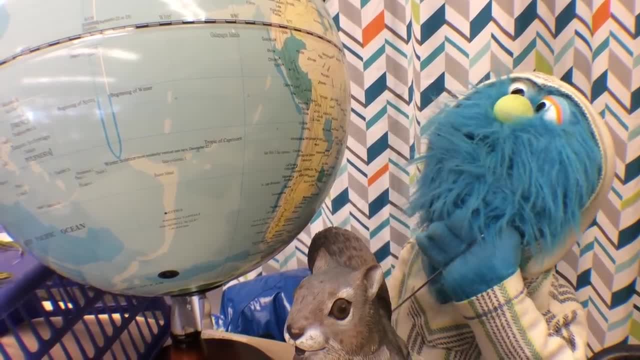 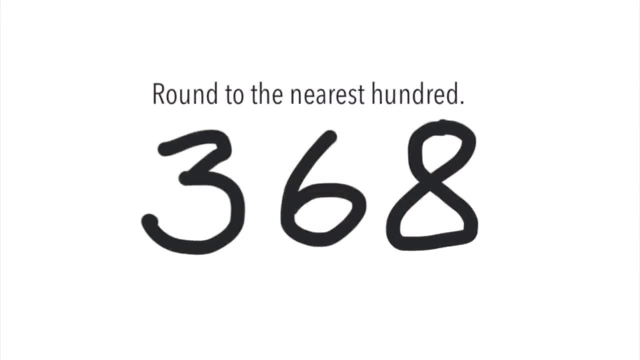 Okay, one more problem. Let's try 368.. All right, here we go. So we read the directions and they say round to the nearest hundred. So we underline the number in the hundreds place circle, the number next to it. 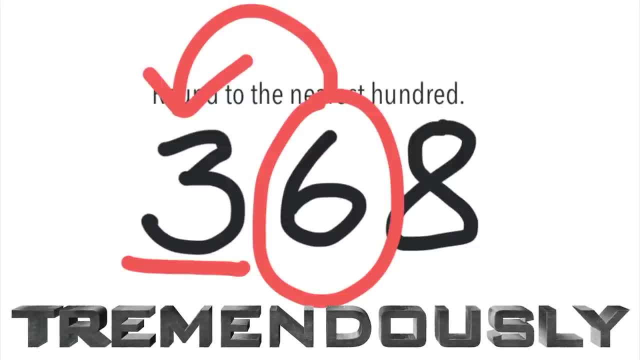 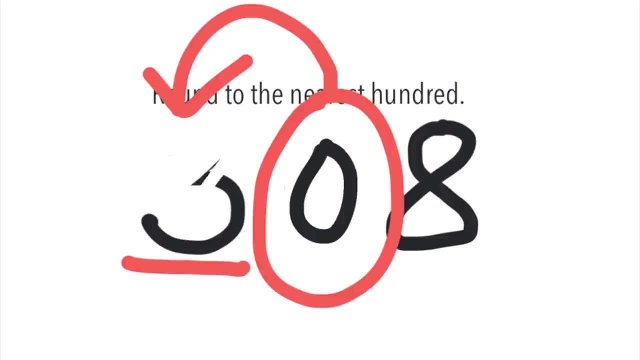 The number we circled affects the other number tremendously. Now we ask ourselves a question: Is the 6 closer to 10 or 0?? Well, it's closer to 10.. So we turn the 6 into a 0, and the other number goes up by 1 and becomes a 4.. 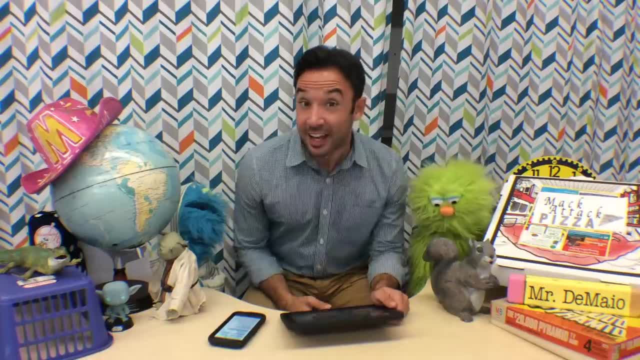 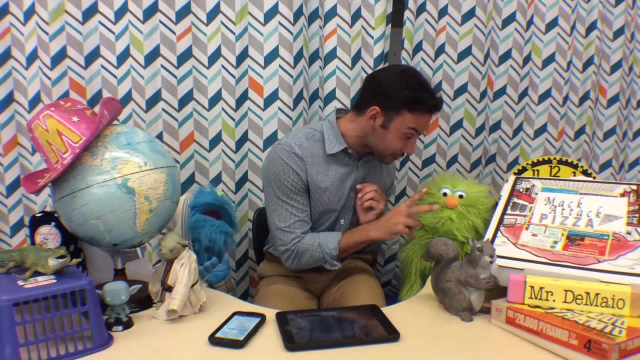 But what about the 8?? It turns into a 0 because it's so lowly. You had to do it, didn't you? When he get worried and pass with the two 6, he said, oh, he's so lowly. 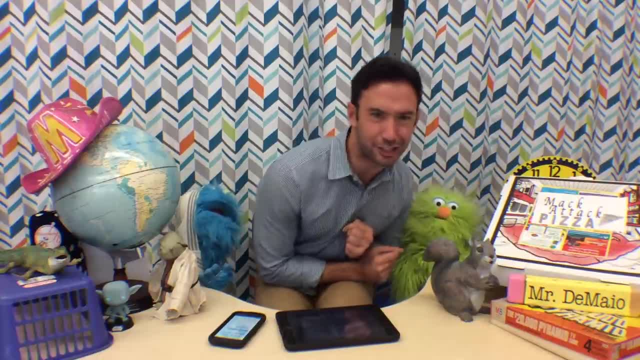 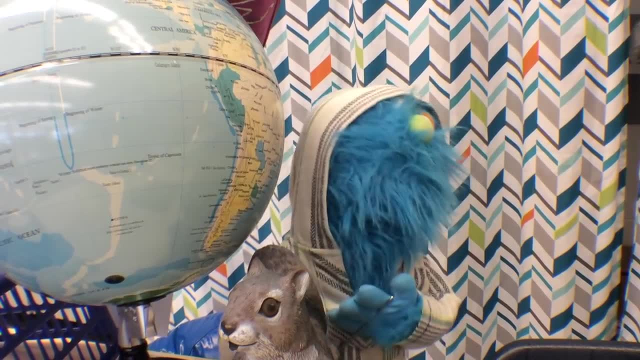 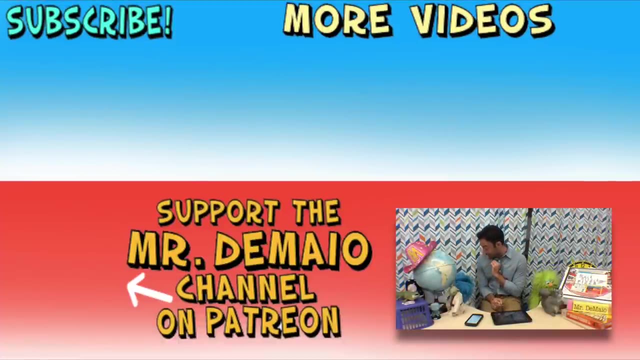 with no one else to him because he's so lowly. Kids, it's not too late to change the channel. Do it, Do it. Lowly. It could have suffered a lunar night with no one else For a plane ticket. 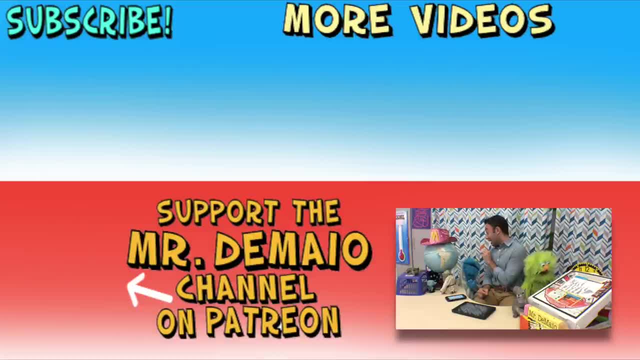 Not easy one. Not easy one but a plane ticket And you have one seat and one popcorn, because he's really lowly.